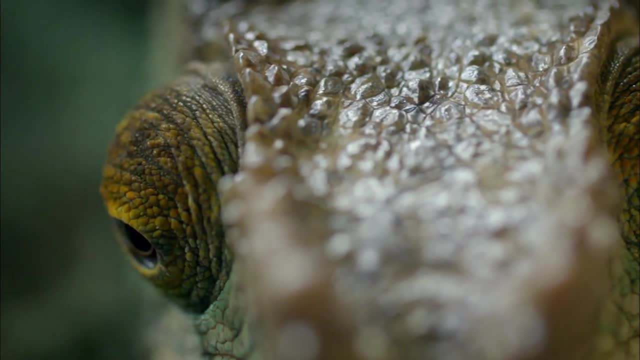 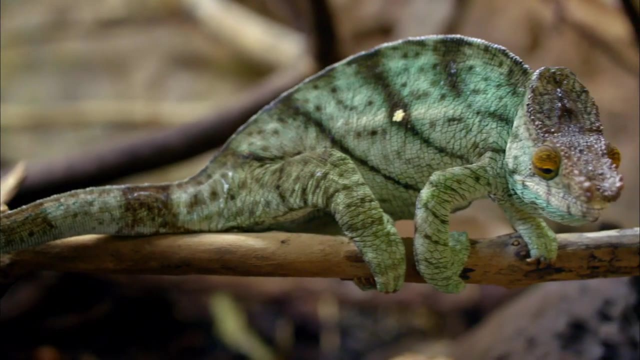 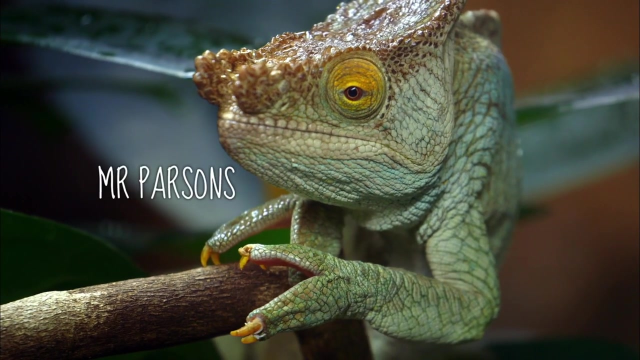 Ready for your breakfast, You hungry. Mr Parsons is a really lovely animal. He definitely needs like the full official title of Mr Parsons. I think anything else wouldn't do him justice. Mr Parsons is a chameleon whose wild counterparts hail from Madagascar. 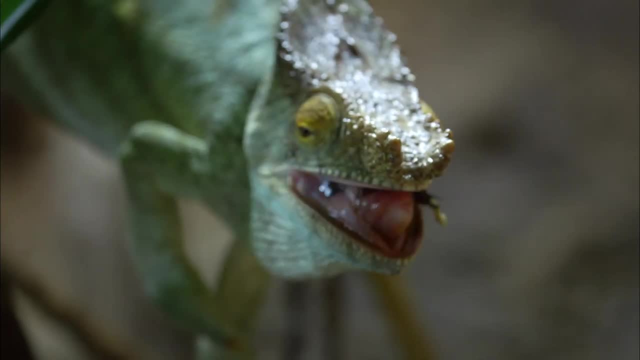 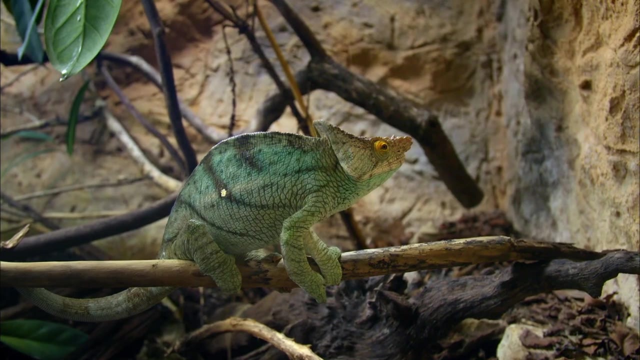 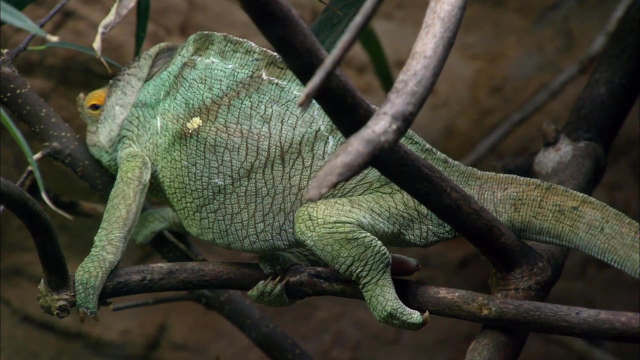 Good boy. Chameleons generally are very easily stressed. They're kind of treading the thin line of being like happy one minute and then suddenly change in temperature, change in keeper, any kind of disturbance at all, and their colours will change. 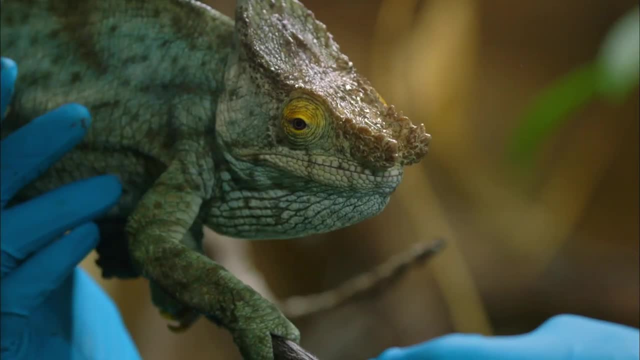 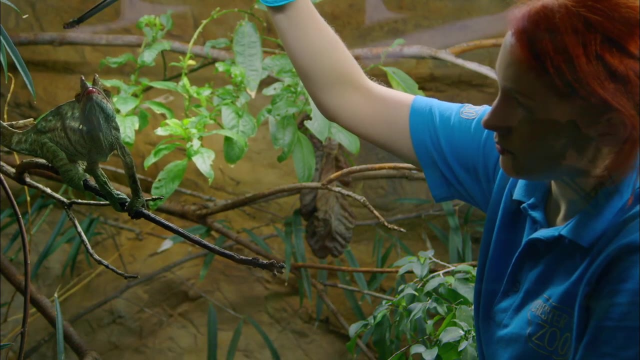 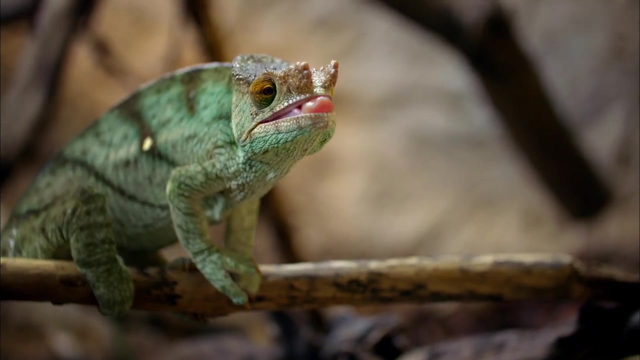 But Mr Parsons is actually. he's a proper gentleman. He won't go dark coloured and puff up and hiss like your average chameleon would Like you go in and you feed him and he doesn't just take off afterwards. he'll hang around and I like to think it's you know him, kind of saying his little thank yous. 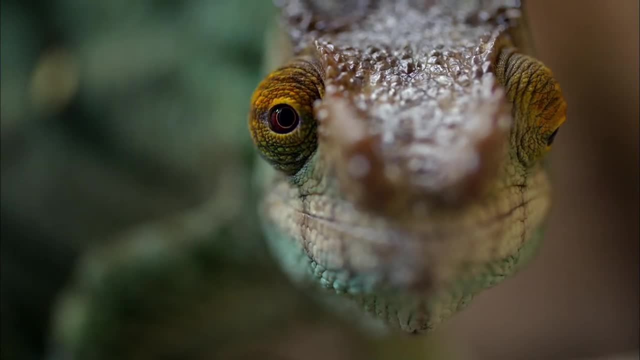 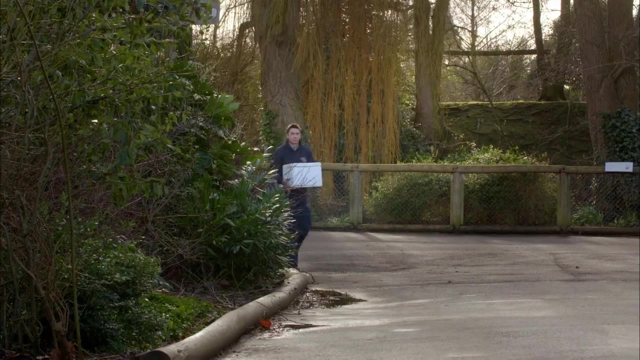 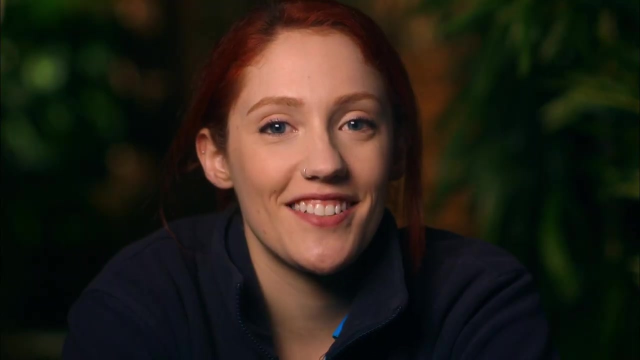 Despite Mr Parsons being so eligible. he's been single for the last year, But this could be about to change, as Daphne has just arrived from a zoo in Paris to meet him. I think Mr Parsons is really lovable. I don't know how anybody couldn't love him. 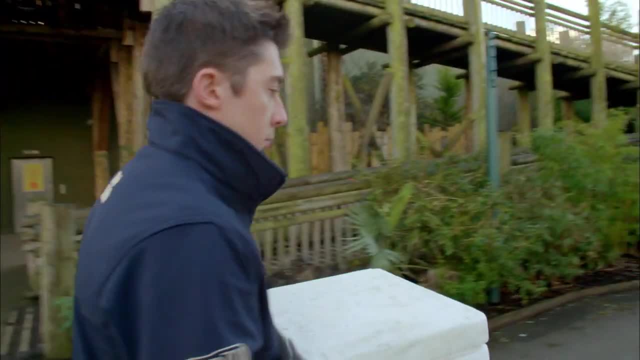 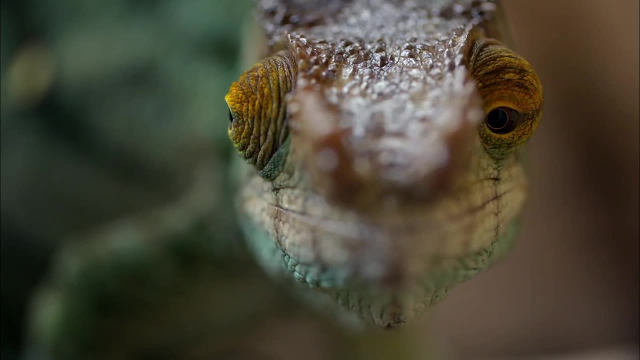 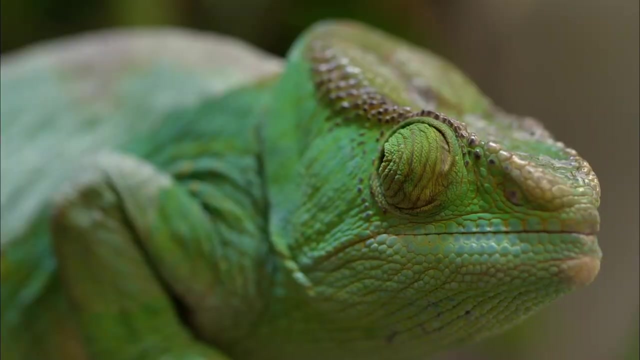 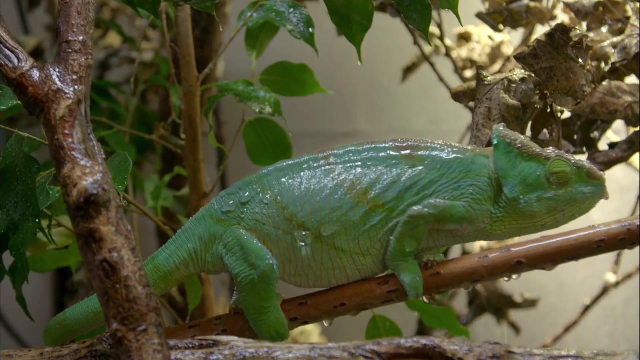 You know he's fairly happy having the bachelor life, but I think it'd be a real shame not to give him the opportunity to have some little Parsons. In the quarantine section of the reptile house the keepers are playing cupid. Daphne has just arrived from Paris and is being lined up for Mr Parsons. 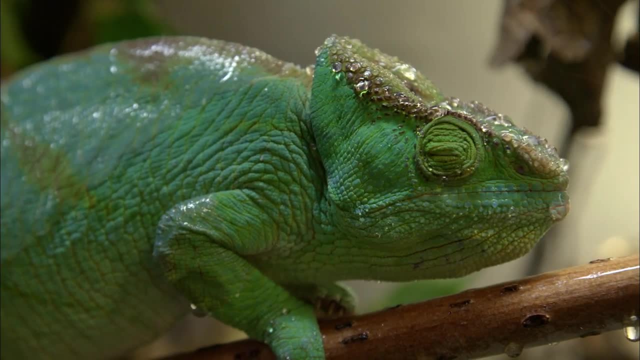 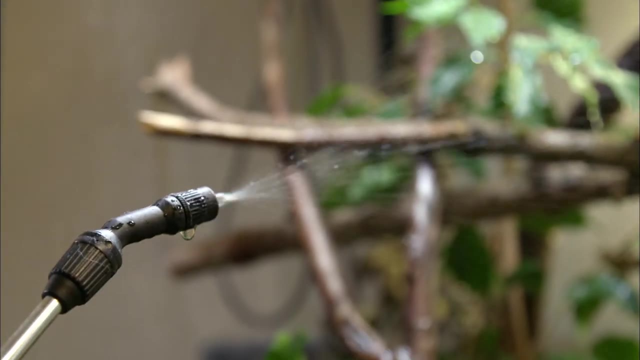 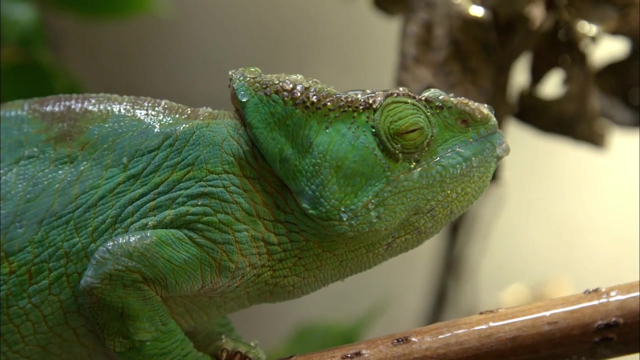 Chameleons don't like to drink still water. They prefer droplets that fall from leaves and branches when it rains. In the zoo they try to replicate this. They try to replicate that with a hose. She seems really chilled out. 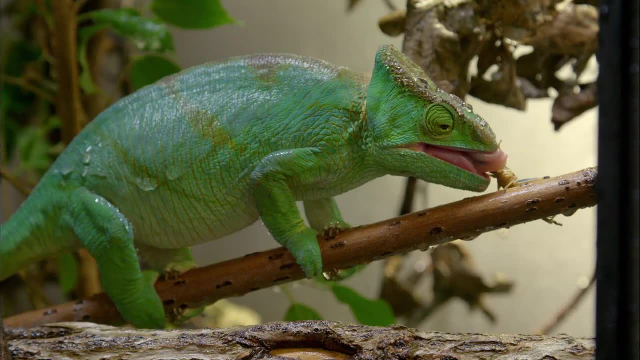 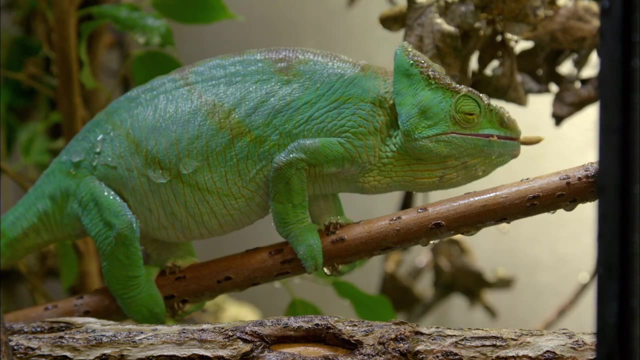 Travelling can be stressful for anybody, never mind chameleons. She's a really nice, big, chunky female, which is exactly what you want in a chameleon Females- really. it's the bigger the better, so we're really pleased with her.